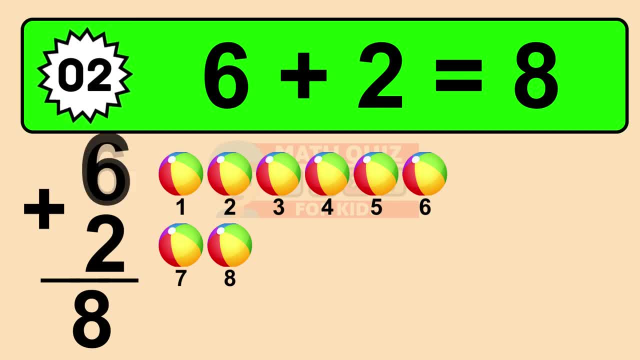 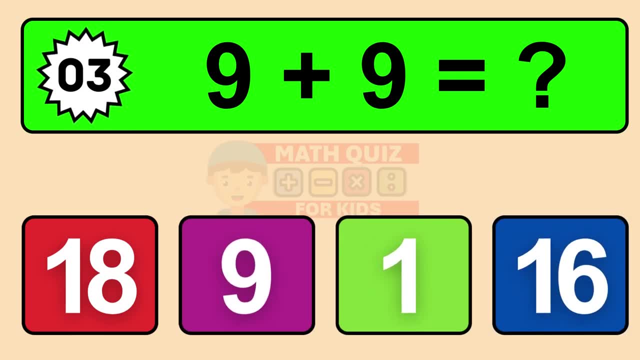 So the answer is: 6 plus 2 is 8.. Let's count it 1,, 2,, 3,, 4,, 5,, 6,, 7, 8.. Question 3. 9 plus 9 equals what? 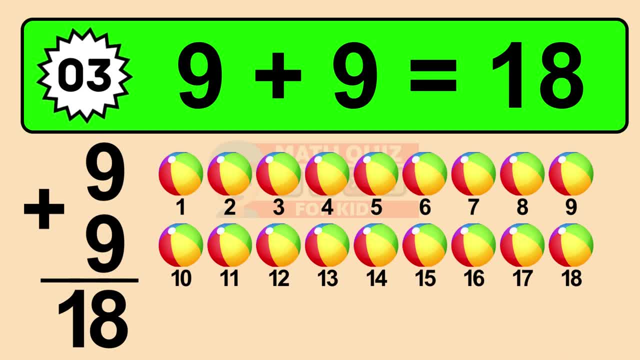 So the answer is 9 plus 9 is 18.. Let's count it 1,, 2,, 3,, 4,, 5,, 6,, 7,, 8,, 9,, 10,, 11,, 12,, 13,, 14,, 15,, 16,, 17,, 18.. 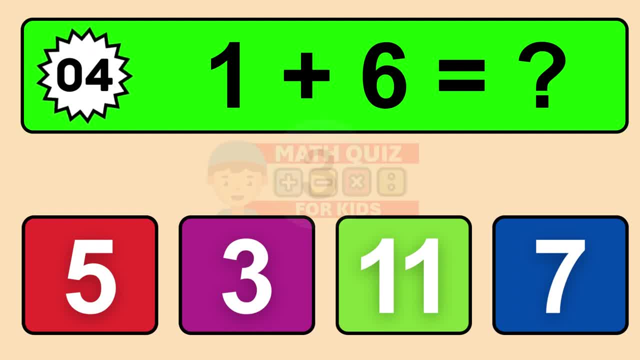 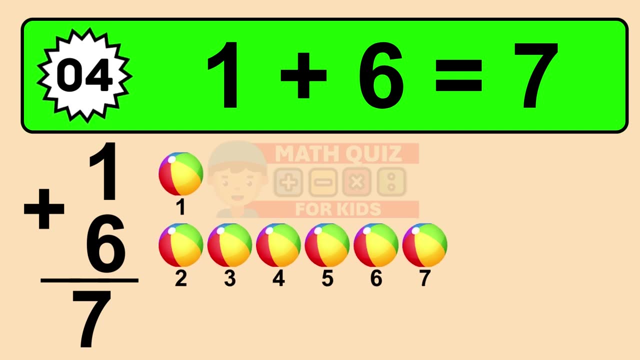 Question 4.. 1 plus 6 equals what So? the answer is: 7 plus 9 equals what So? the answer is: 1 plus 6 is 7.. Let's count it: 1,, 2,, 3,, 4,, 5,, 6,, 7.. 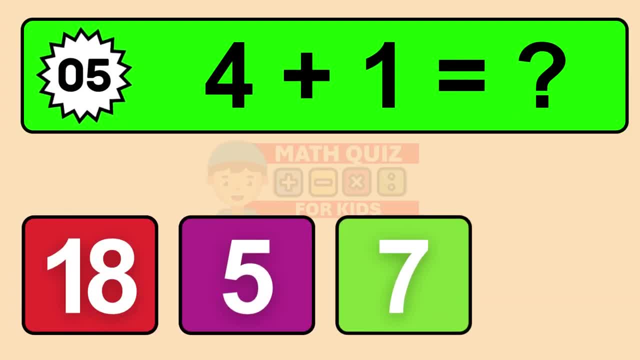 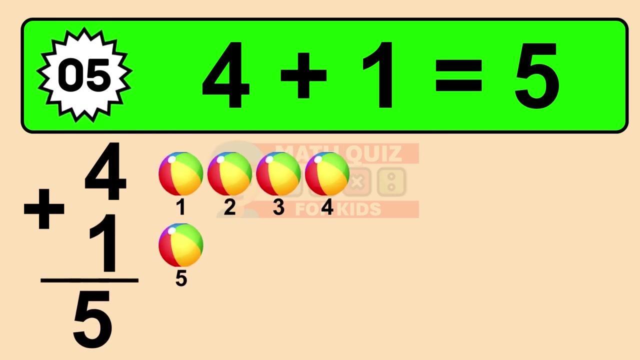 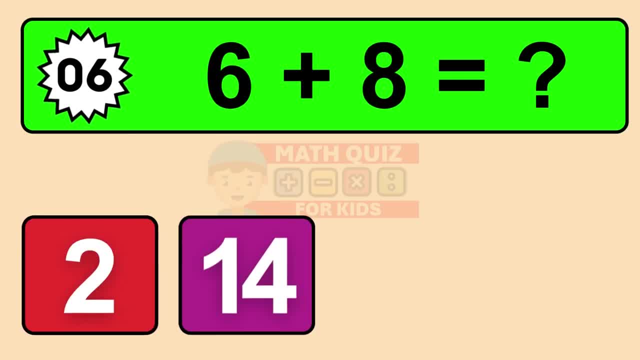 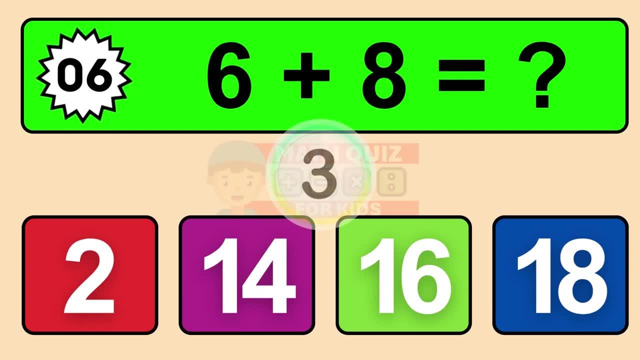 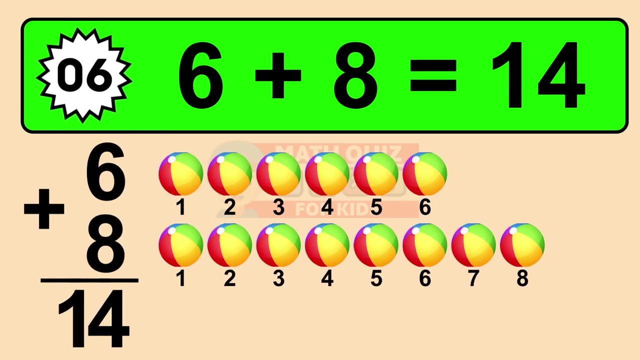 question: 6, 6 plus 8 equals what. so the answer is: 6 plus 8 is 14. let's count it 1, 2, 3, 4. let's count it 1, 2, 3, 4, 5. so the answer is: 6 plus 8 is 14. let's count it 1, 2, 3, 4. 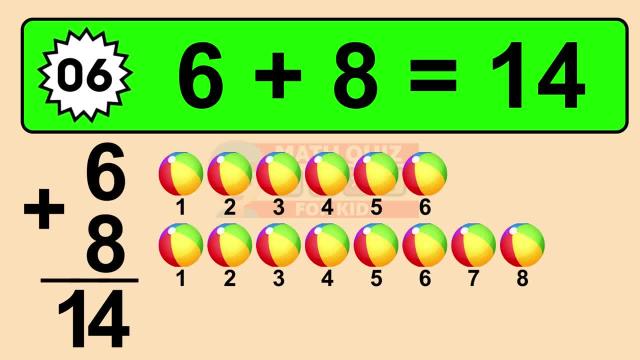 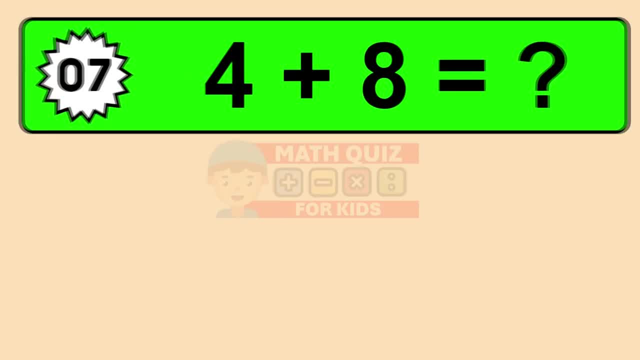 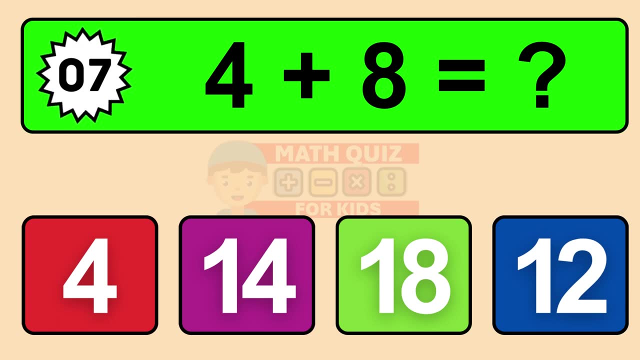 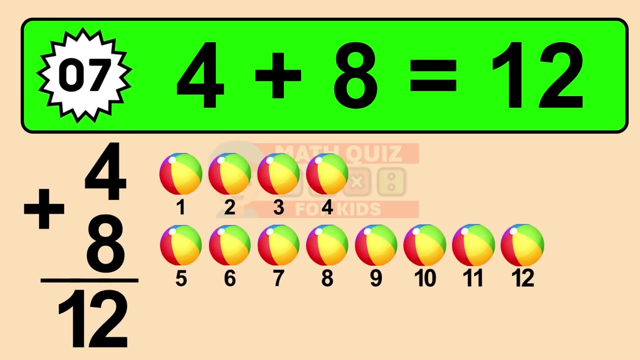 5, 6, 7, 8, 9, 10, 11, 12, 13, 14. question: 7, 4 plus 8 equals what so? the answer is: 6 plus 8 is 14. let's count it: 1, 2, 3, 4, 5, 6, 7, 8, 9, 10, 11, 12. 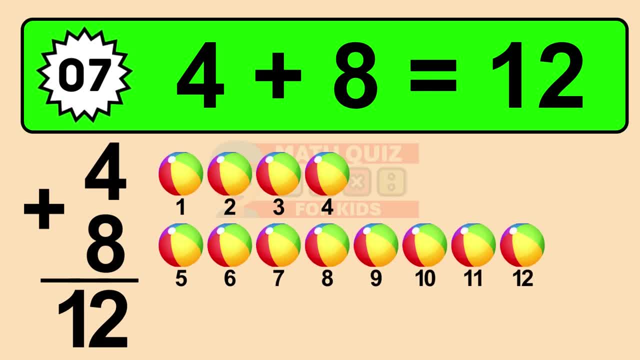 so the answer is: 6 plus 8 is 14. let's count it 1, 2, 3, 4, 5, 6, 7, 8, 9, 10, 11, 12. so the answer is: 6 plus 8 is 14. let's count it: 1, 2, 3, 4, 5, 6, 7, 8, 9, 10, 11, 12. 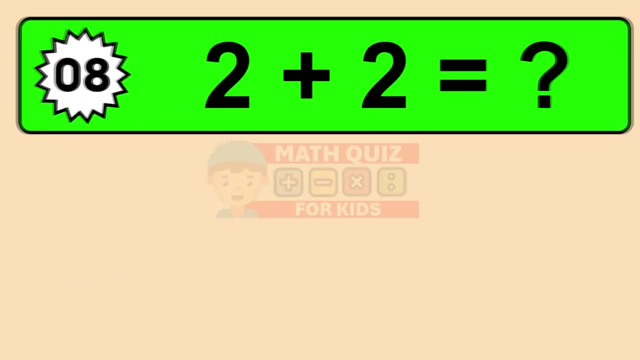 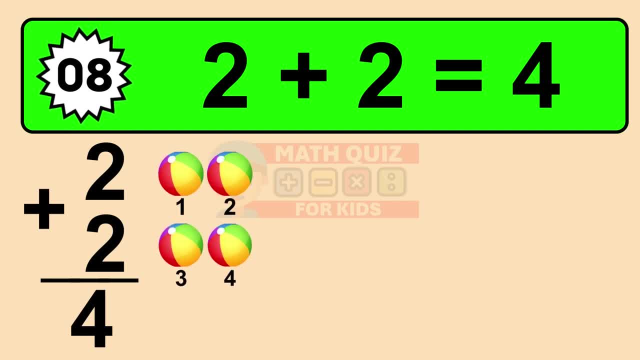 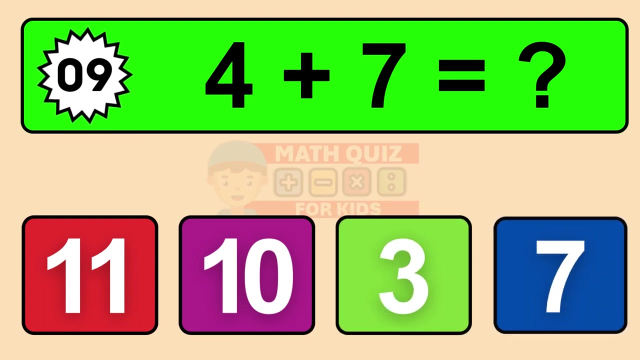 so the answer is 6 plus 8 is 14. let's count it: 1, 2, 3, 4, 5, 7, 8, 10, 12, 16, 16, 16, 17, 18. leaked question nine four plus seven equals. question nine four plus seven equals. 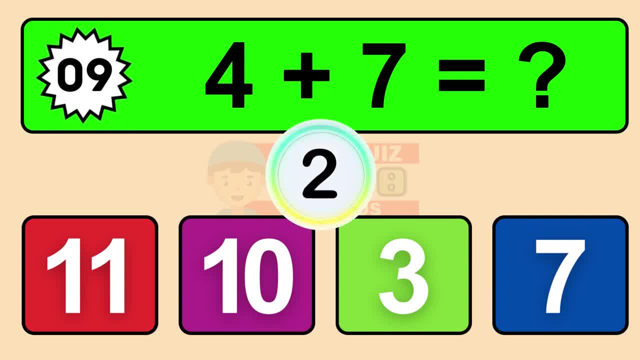 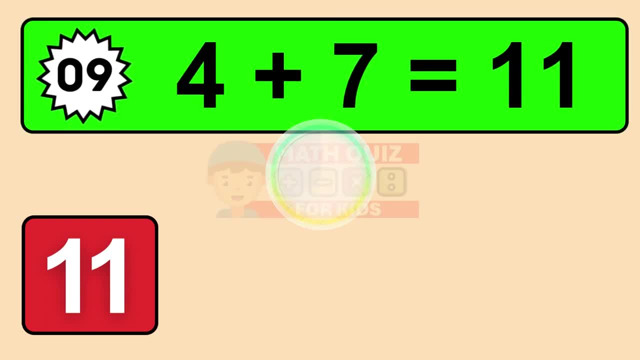 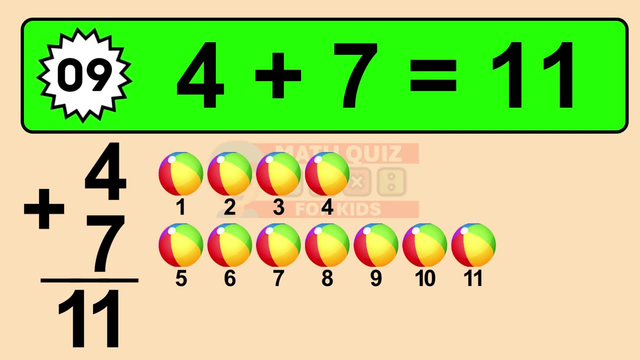 what, what? So the answer is: 4 plus 7 is 11.. Let's count it: 1,, 2,, 3,, 4,, 5,, 6,, 7,, 8,, 9,, 10,, 11.. 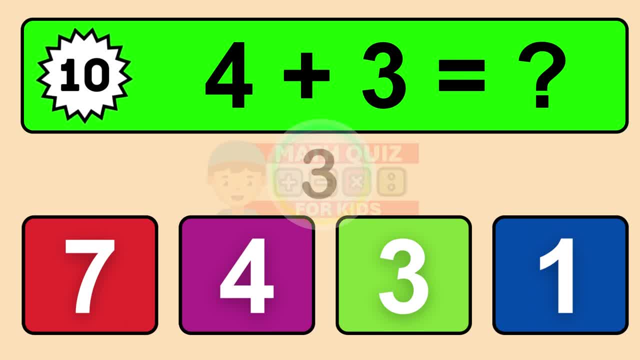 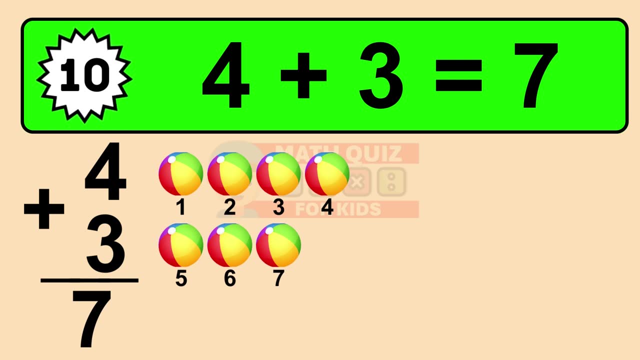 Question 10.. 4 plus 3 equals what? So the answer is: 4 plus 3 is 7.. Let's count it: 1,, 2,, 3,, 4,, 5,, 6,, 7.. 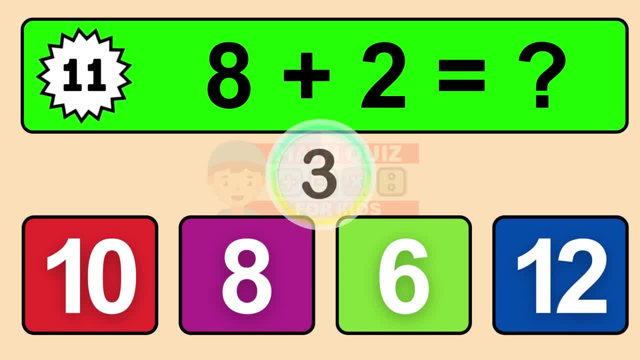 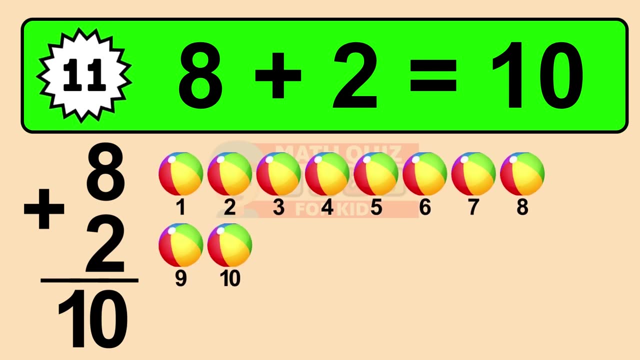 Question 11.. 8 plus 2 equals what? So the answer is: 8 plus 2 is 10.. Let's count it: 1,, 2,, 3,, 4,, 5,, 6,, 7,, 8,, 9,, 10.. 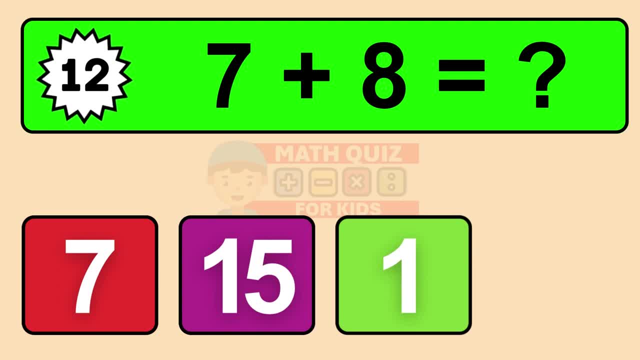 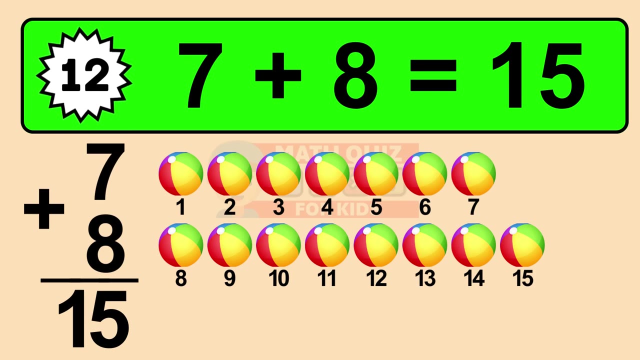 Question 12.. 7 plus 8 equals what? So the answer is: 7 plus 8 is 15.. Let's count it: 1,, 2,, 3,, 4,, 5,, 6,, 7,, 8,, 9,, 10.. 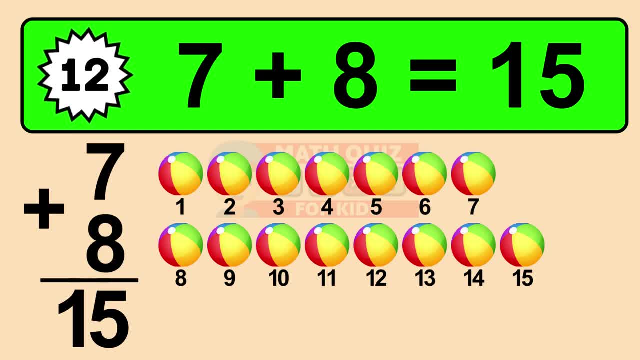 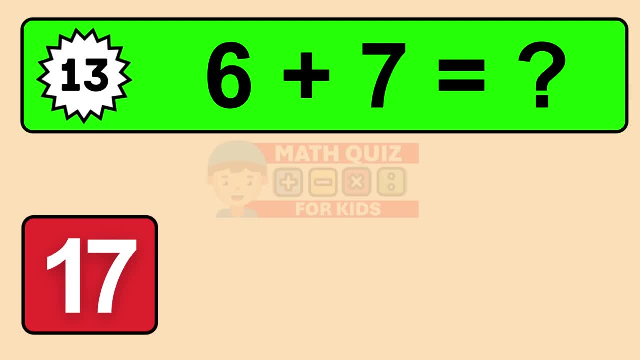 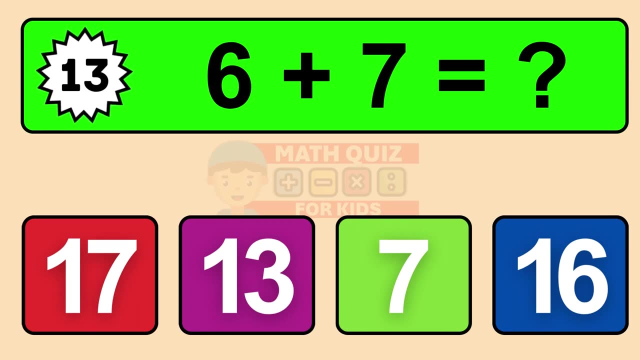 5,, 6,, 7,, 8,, 9,, 10,, 11,, 12,, 13,, 14, 15.. Question 13. 6 plus 7 equals what? Question 13. 6 plus 7 equals what. 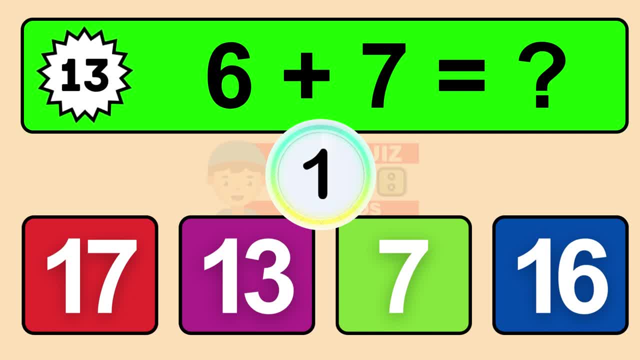 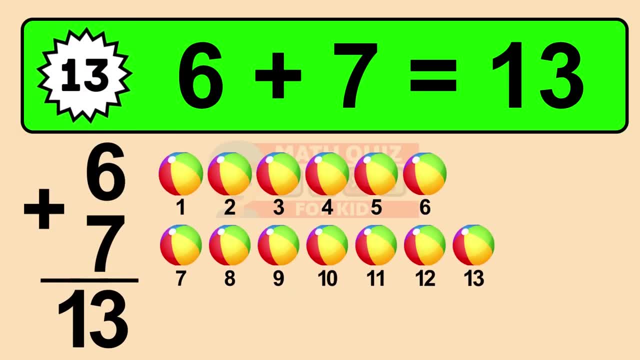 So the answer is: 6 plus 7 equals what? So the answer is: 6 plus 7 is 13.. Let's count it: 1,, 2,, 3,, 4,, 5,, 6,, 7,, 8,, 9,, 10,, 11,, 12,, 13.. 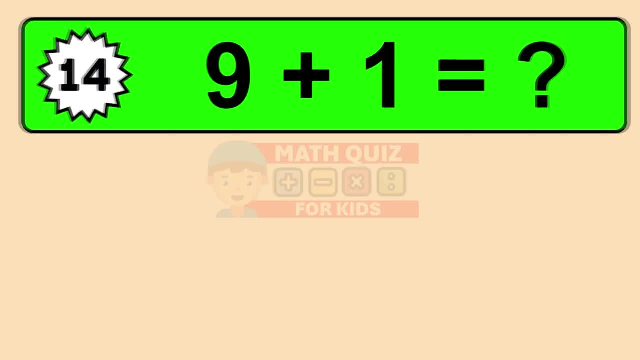 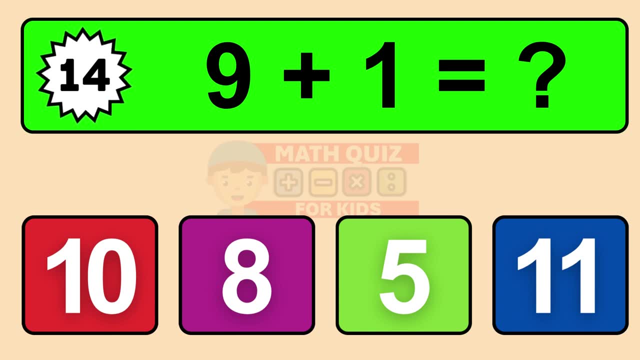 Question 14.. 9 plus 1 equals what? So the answer is: 6 plus 7 is 13.. Let's count it: 1,, 2,, 3,, 4,, 5,, 6,, 7,, 8,, 9,, 10,, 11,, 12,, 13.. 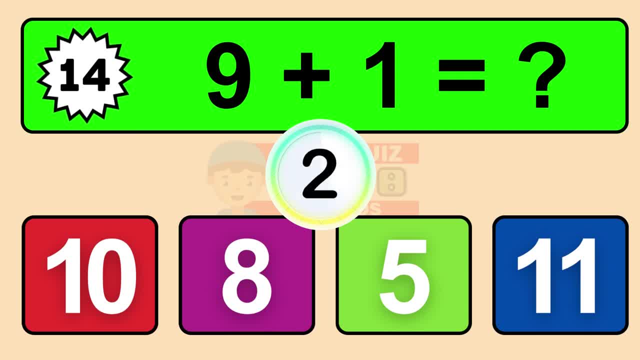 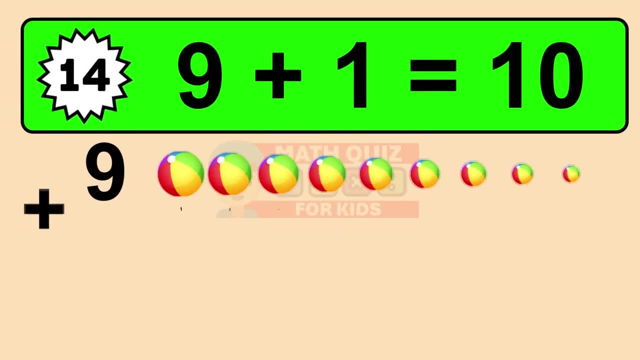 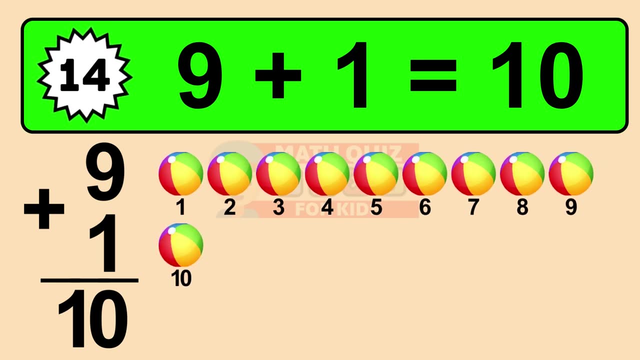 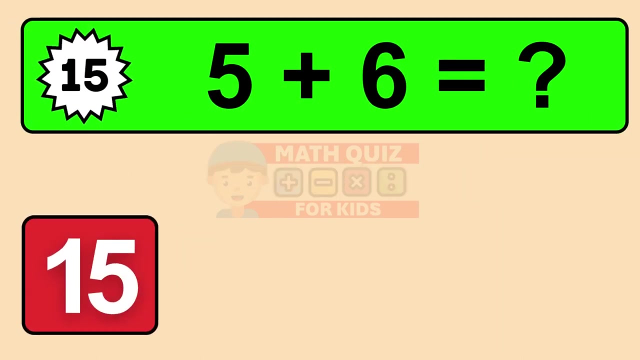 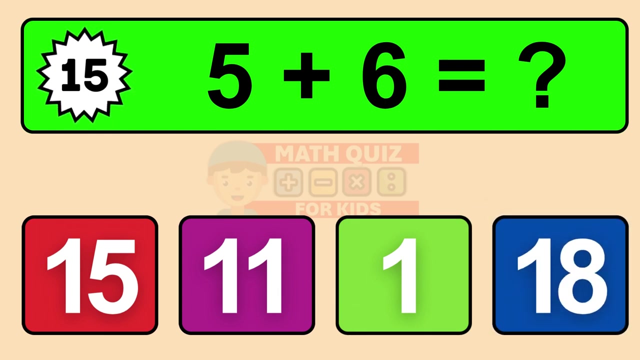 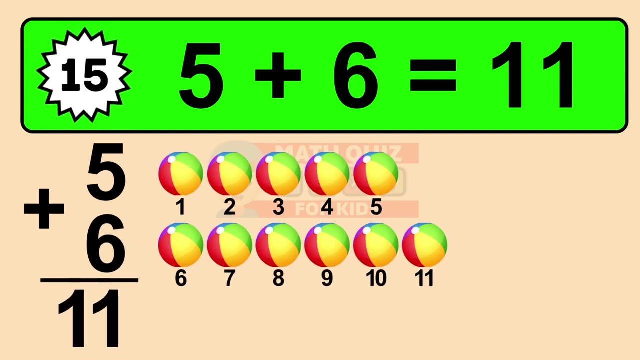 Question 14.. so the answer is: nine plus one is ten. let's count it one, two, three, four, five, six, seven, eight, nine, ten. question 15: 5 plus 6 equals what? so? the answer is: 5 plus 6 is 11. let's count it 1, 2, 3, 4, 5, 6, 7. 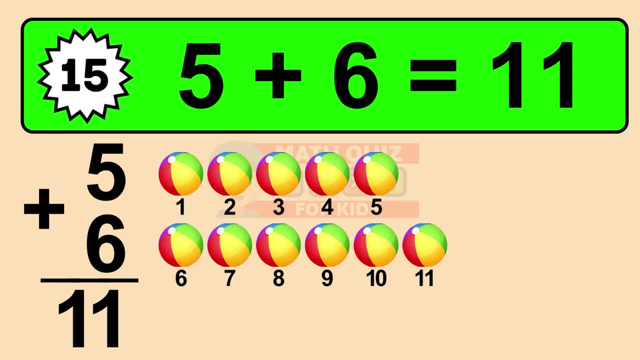 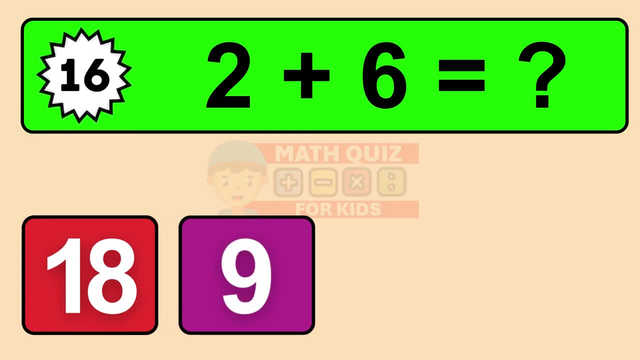 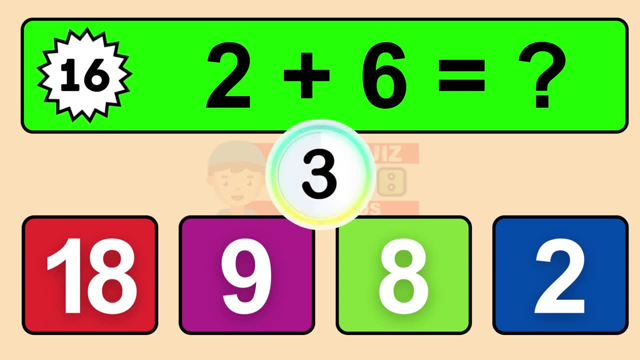 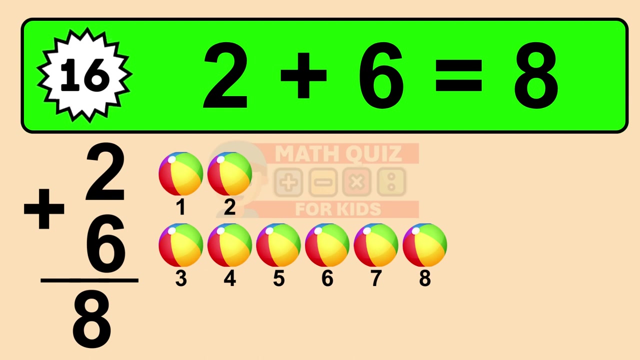 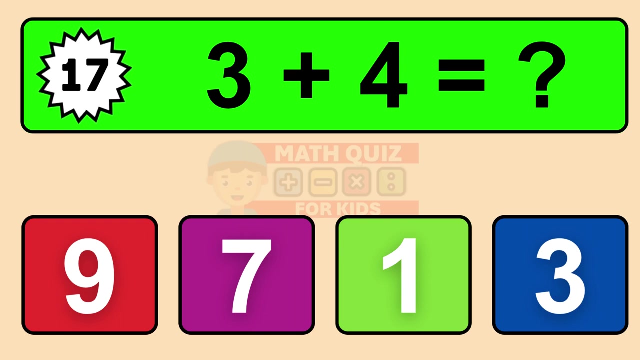 8, 9, 10, 11. question 16: 2 plus 6 equals what. so the answer is is: 2 plus 6 is 8.. Let's count it: 1,, 2,, 3,, 4,, 5,, 6,, 7,, 8.. 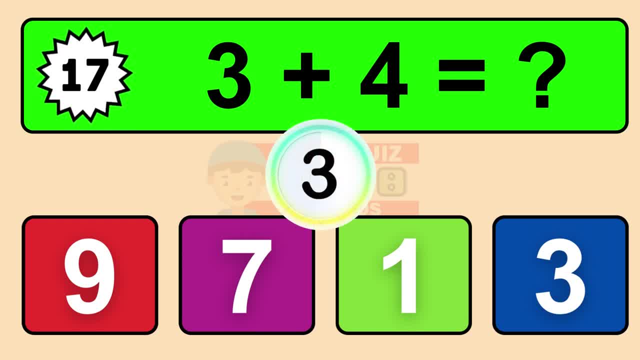 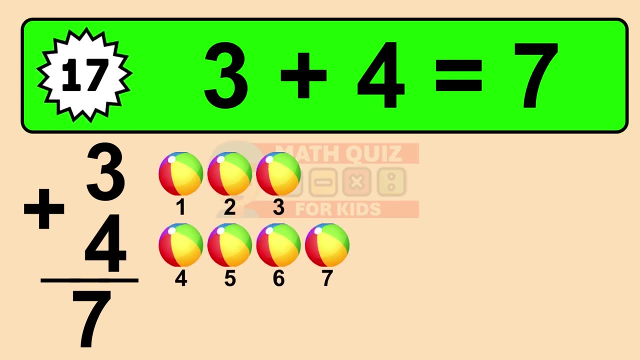 Question 17.. 3 plus 4 equals what? So? the answer is: 3 plus 4 is 7.. Let's count it: 1,, 2,, 3,, 4,, 5,, 6,, 7.. 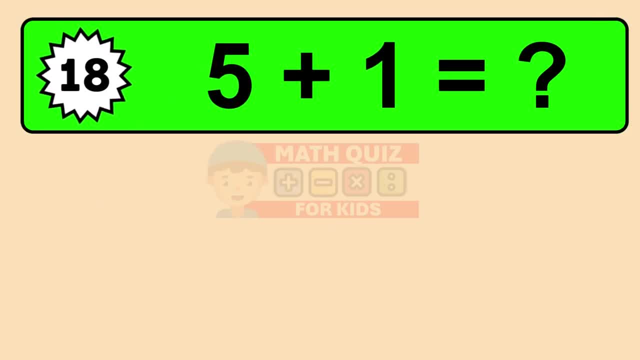 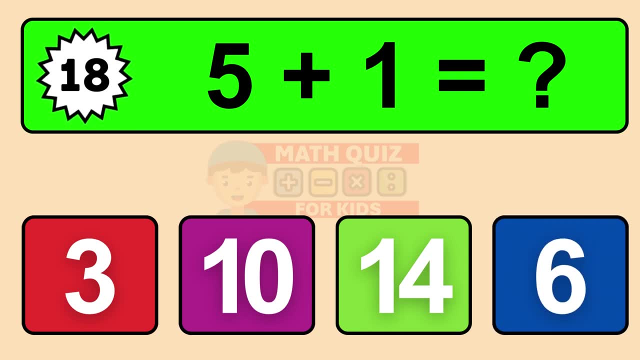 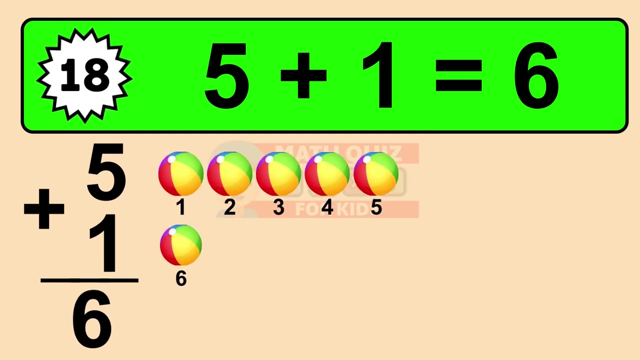 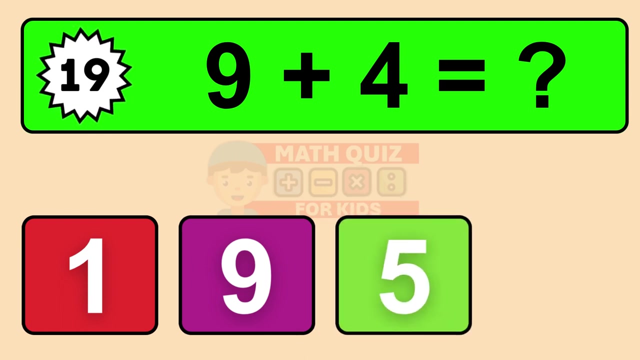 Question 18.. 5 plus 1 equals what. So the answer is: 5 plus 1 is 6.. Let's count it: 1,, 2,, 3,, 4,, 5, 6.. Question 19.. 9 plus 4 equals what. 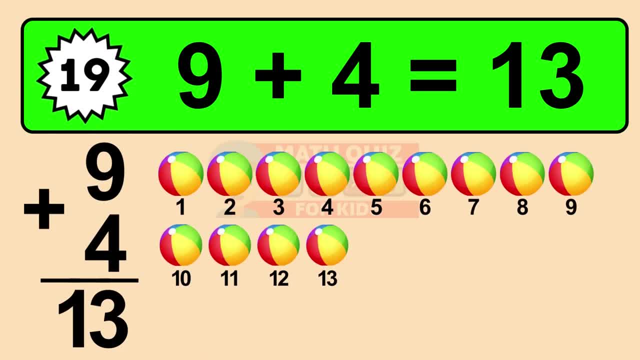 So the answer is 9 plus 4 is 13.. Let's count it 1,, 2,, 3,, 4,, 5,, 6,, 7,, 8,, 9,, 10,, 11,, 12,, 13.. 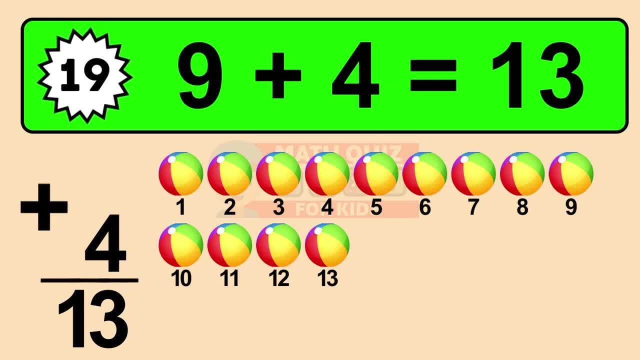 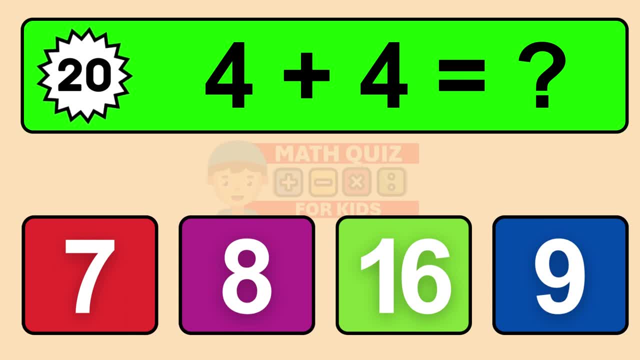 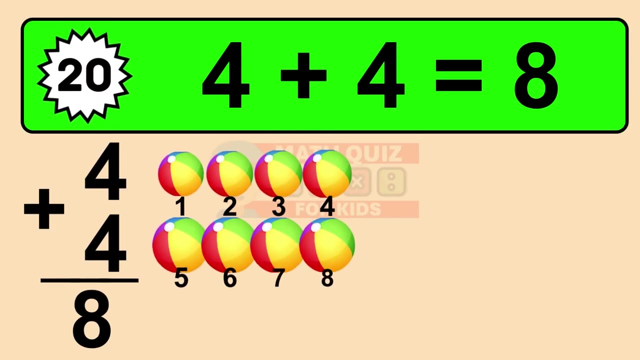 Question 20.. 4 plus 4 equals what? So the answer is: 4 plus 4 is 8.. Let's count it: 1,, 2,, 3,, 4,, 5,, 6,, 7,, 8.. 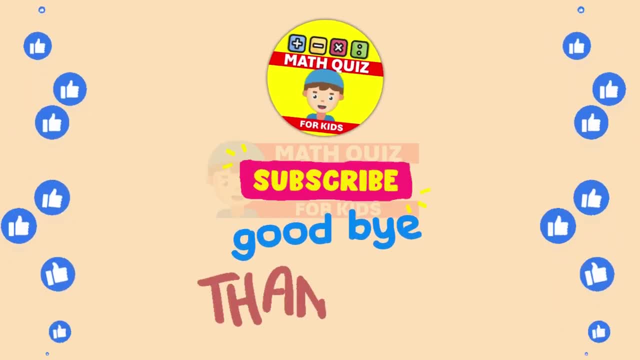 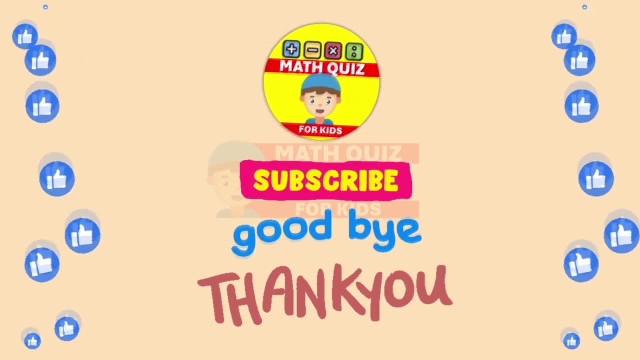 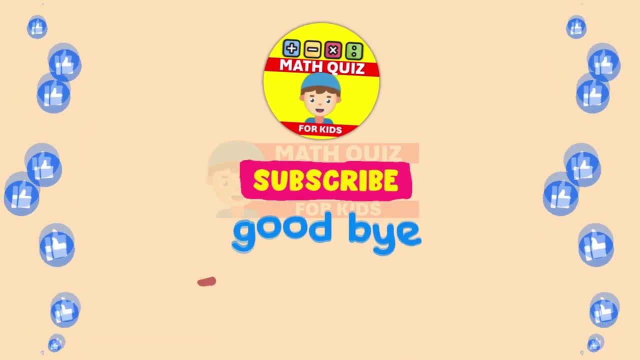 How many did you get right? We bet you did awesome. Remember: practice makes perfect. Don't forget to click the like button if you had fun and subscribe so you can join us for even more math quiz adventures. Let's keep the math magic alive. 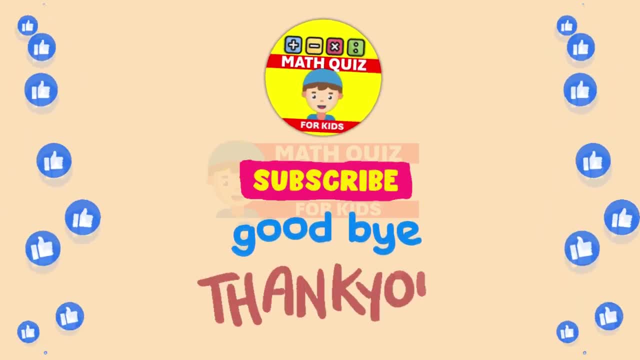 We'll see you next time. Bye.